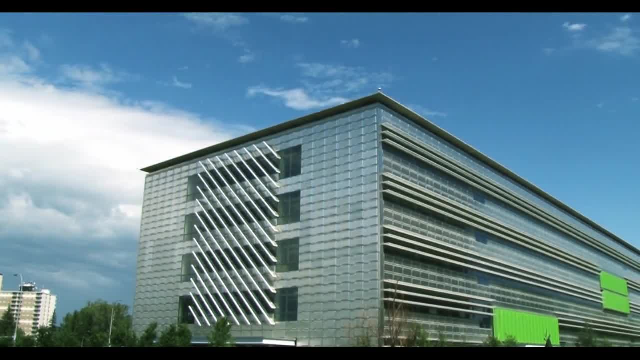 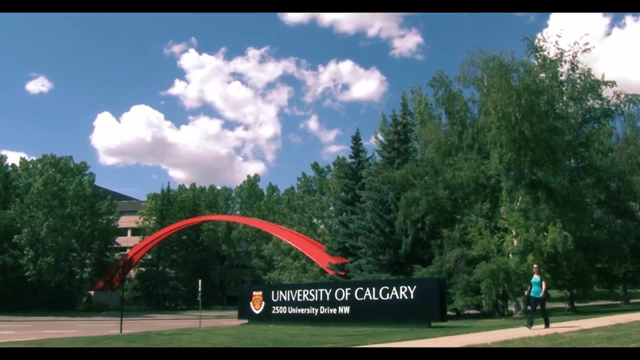 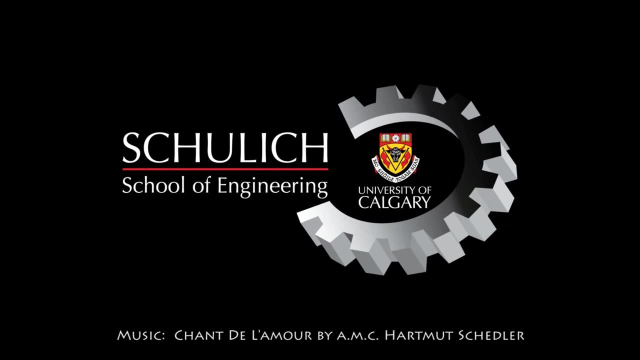 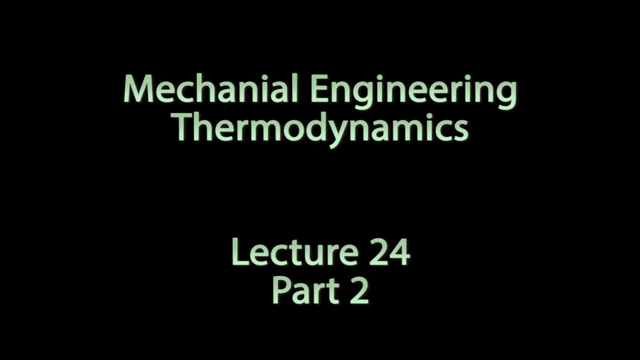 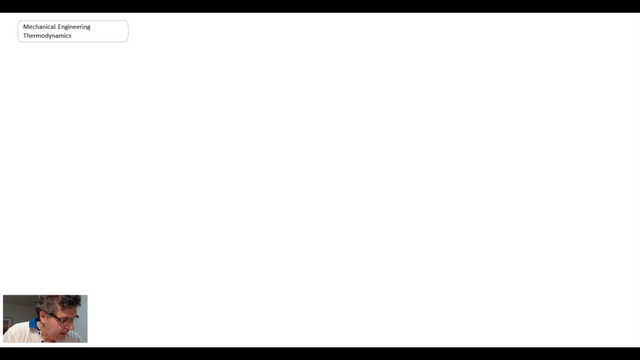 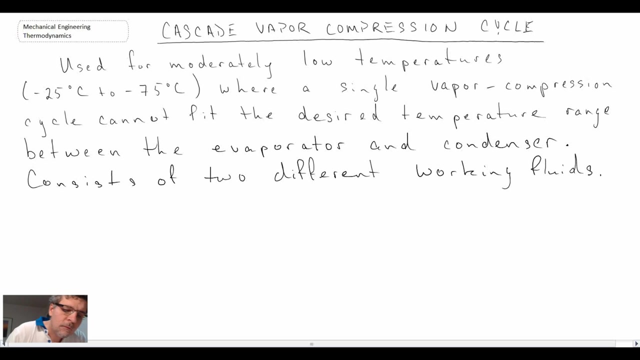 The first more industrial refrigeration system that we're going to look at is going to be the cascade cycle or the cascade vapor compression cycle. So the cascade vapor compression cycle is one whereby we have two different working fluids. Essentially, what we have is two refrigeration systems, one sitting on top of another, And the reason why we have two working 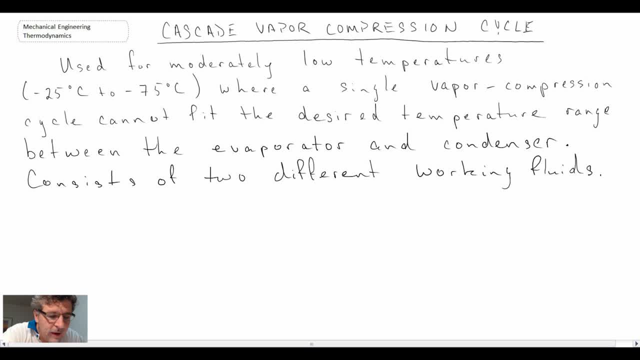 fluids is to enable us to get to lower temperatures than we could get to with just a single working fluid, And consequently the fluids would be selected carefully, ensuring that we can get down to lower temperatures, And this is for what we would call moderately low temperatures. We're 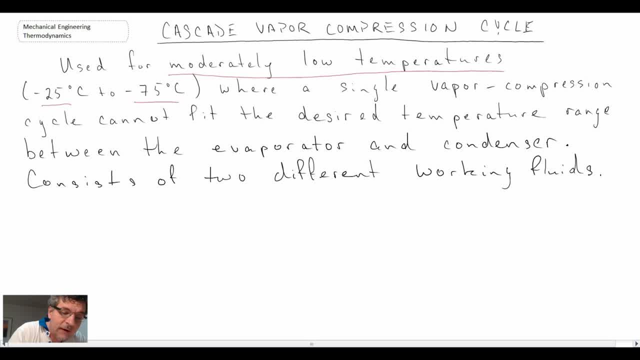 not looking at cryovoltaics, We're looking at low temperatures. We're looking at low temperatures, But we're looking at things minus 25 to minus 75 degrees C. That would be very difficult with our 134A And consequently you have two different working fluids here, And what we'll do is we'll 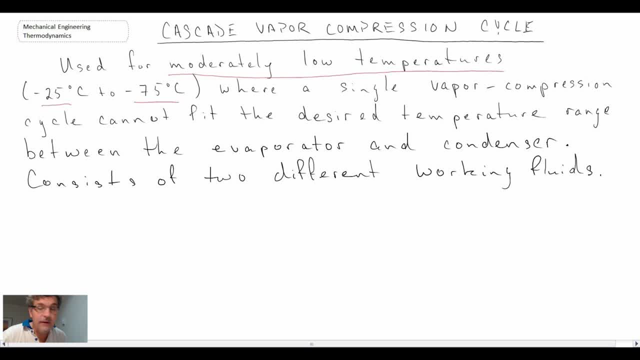 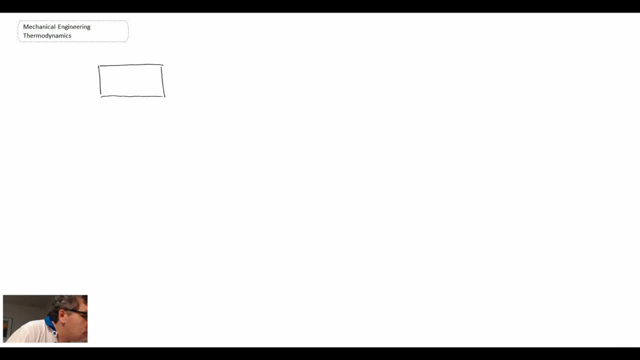 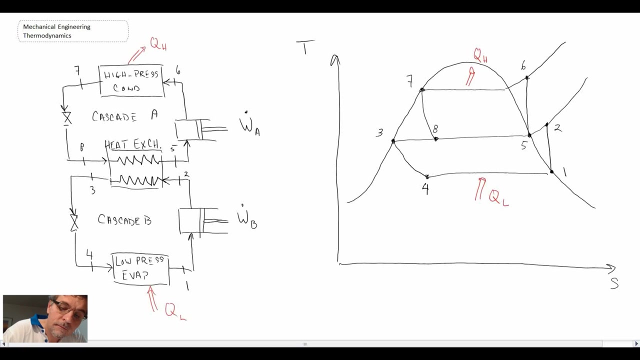 begin by looking at the process diagram and schematic, And then I'll write out an equation that shows us how to determine the coefficient of performance for a cascade vapor compression cycle. Thank you. So here we have the process diagram and the process schematic for our cascade refrigeration. 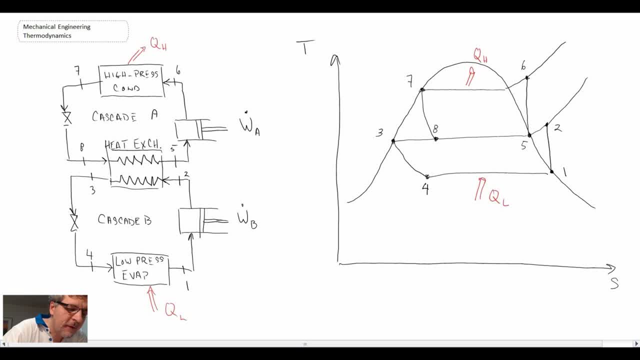 cycle, and the main difference between what we saw before is that we have two compressors- We have compressor A and compressor B, and we have a heat exchanger operating between the two cascades, instead of what we had before with an evaporator. The evaporator is now down at the bottom, and so heat exchange is going on between the two. 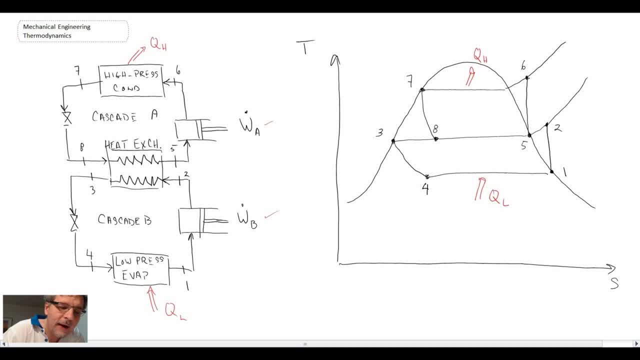 working fluids. When we look at this on a process schematic or in terms of the process diagram, I should say above we have cycle A and then below we would have cycle B. Now, in doing this, we do attain a savings, Mainly in terms of reduced work. 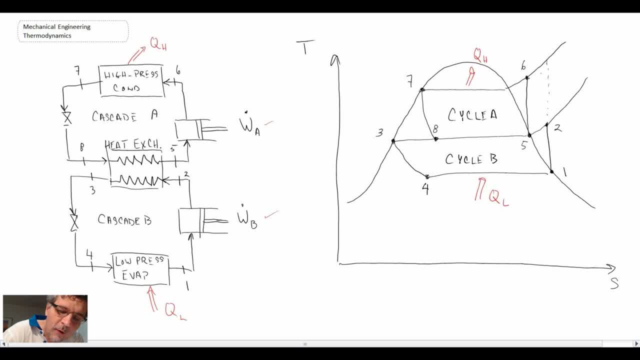 So if we just had a single fluid, we would have to add more work in here, and so this could be considered as being the reduced work And we also attain increased refrigeration, because if we only had the one fluid going through this cycle, the throttling process would bring it down to here somewhere. 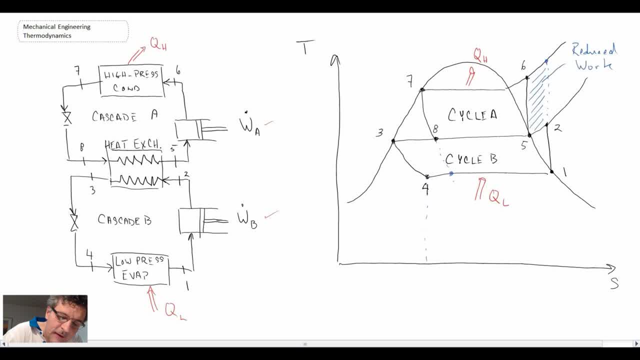 And if we only had one fluid going through this cycle, the throttling process would bring it down to here somewhere, And so the difference between this and this is actually increased refrigeration. So what we're going to do now, we're going to take a look at, basically, the performance. 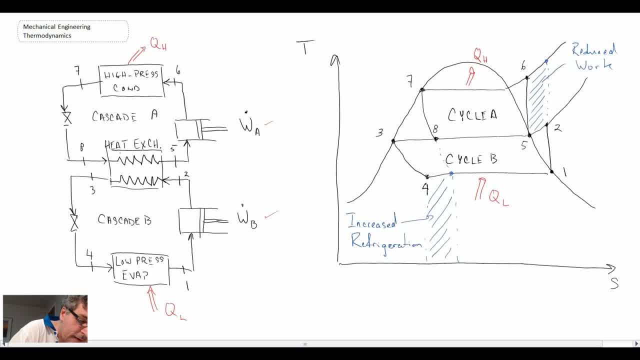 of the heat exchanger where what we have is evaporation- Evaporation Going on here, and on the bottom part we have condensation or the condenser unit. We'll take a look at the heat exchanger and that will enable us to determine the coefficient. 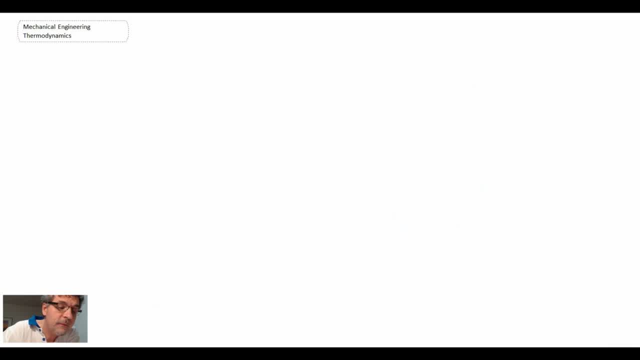 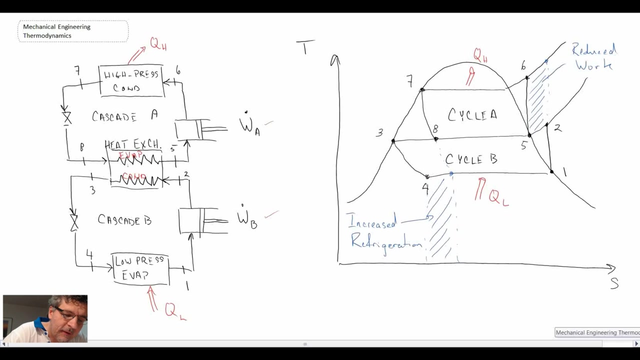 of performance for this cycle. So that's what we'll do next. So, looking at performance of the heat exchanger, what we have is the mass flow rate of fluid from cycle A and the mass flow rate of fluid from cycle B, and we know the change in state.